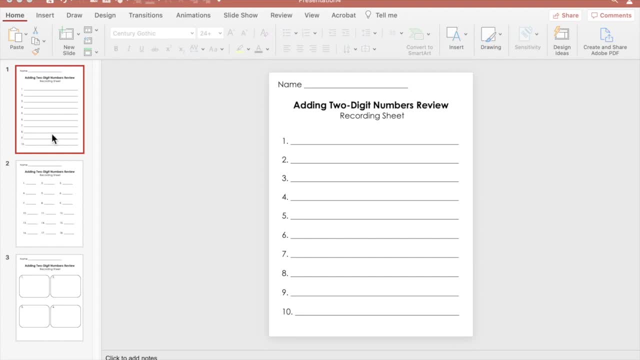 down their answers individually. So we're going to look at three different examples of a recording sheet. So here's one, two with shorter lines and then three where you have more space for them to show their work. Let's get started. So we're going to go to file and start a new presentation. 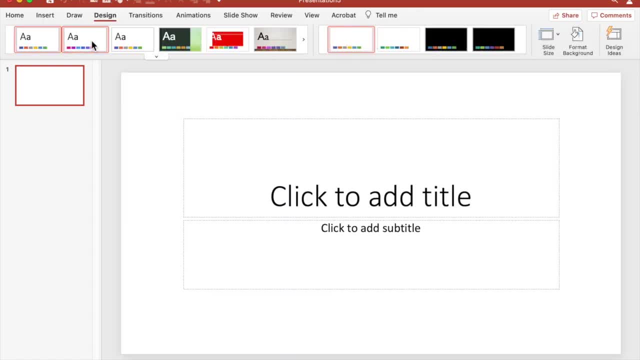 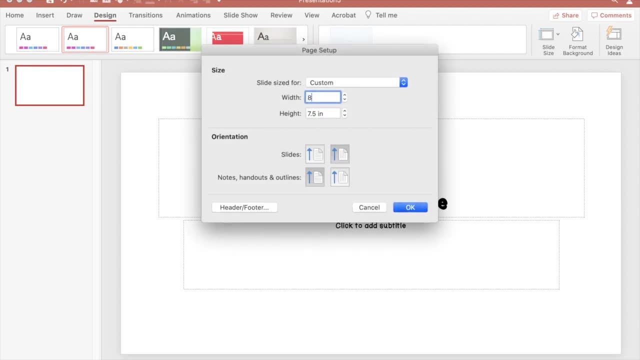 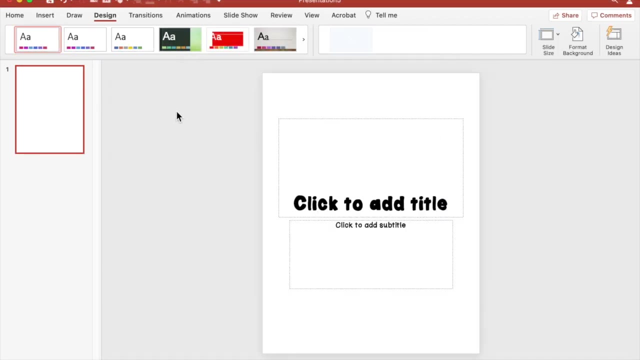 And here I'm going to go to design. click on my default settings, default colors. I'm going to go to slide size. page setup. switch my width to eight and a half inches and my height to 11. And then press scale up. I'm going to select. 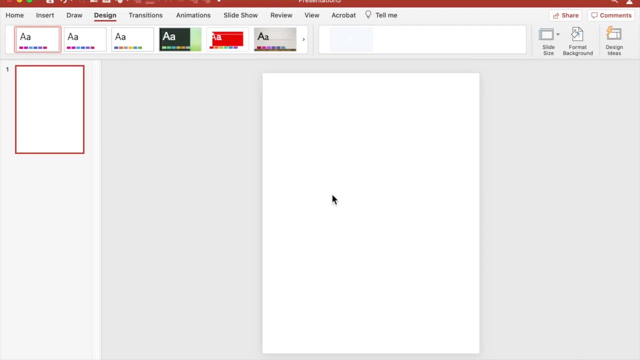 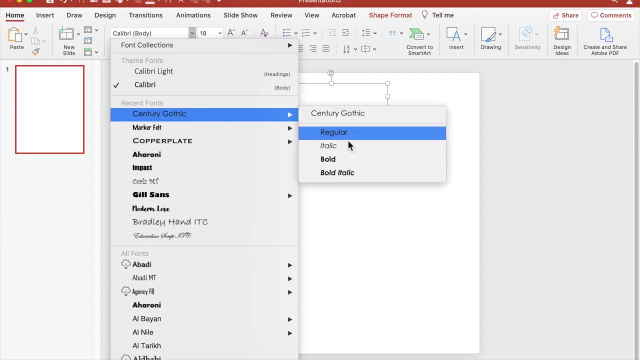 the entire page and delete those default text boxes. So now what I'm going to do is start by inserting a text box to have their name at the top, and I'm going to change the font and the size to a font that I like Regular, and let's do a 24 size. I'm just going to put name and then a long 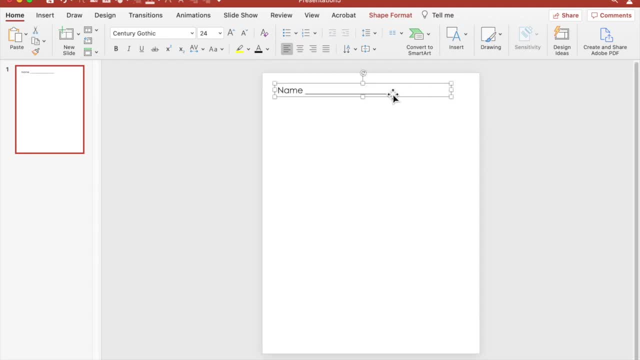 line. I'm using my keyboard, so I'm pressing the shift and the dash key. When you hit shift, it turns the dash key into an underscore, So that's going to be there for their name. I'm going to duplicate that so I can put my title. 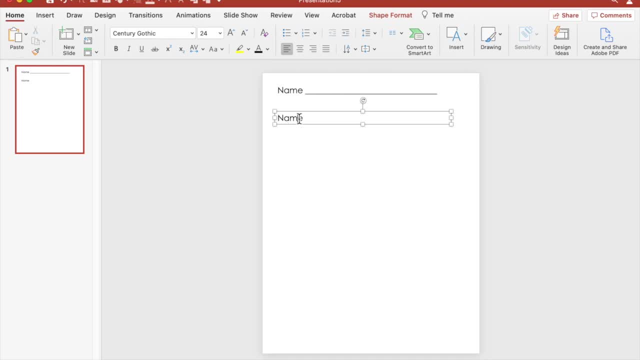 Get rid of the name or get rid of that line, And then I'm going to change this And this can be whatever activity you're working on. You could just put recording sheet so you can make multiple copies. But if you want it to be specific to something, So let's say we have students who are 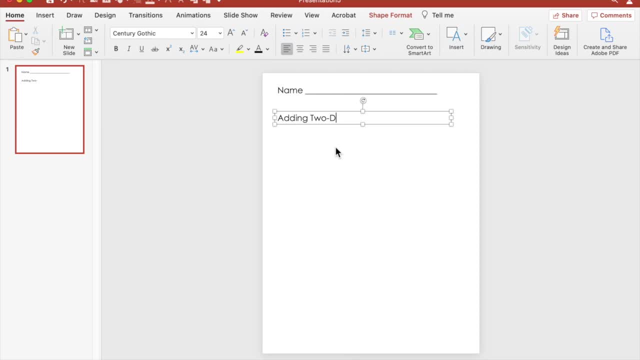 working on adding two digit numbers together And this is a review And this is the recording sheet for that review. So to add a little pop, let's make this bold, center it and then make the size a little bit bigger And then the recording sheet we can put there in the middle. So that works for me. There's the title. 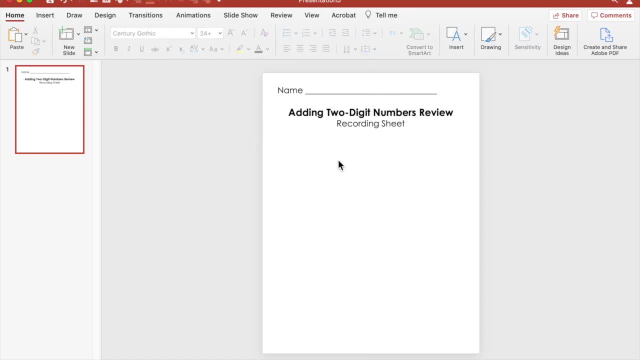 Now, as far as the spaces for them to put their answers, you can add a new text box, or you could have copied the one you already have. Let's change our font And then up our size, So this one's going to be number one, And then I'm just going to put a long 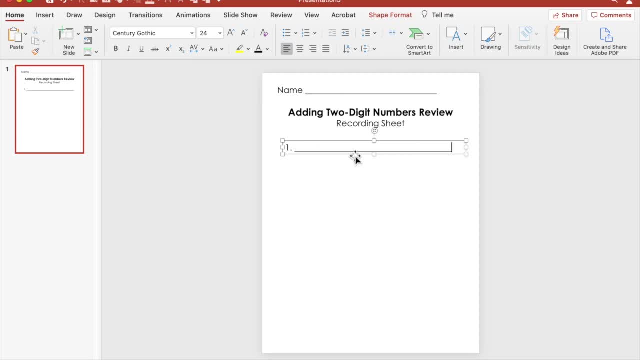 line, using the same technique that I explained before: the shift button and the dash button together. So there's going to be their first answer. Let's move that over just a little bit and we can make this a little longer, And then I'm going to take this text box right click. 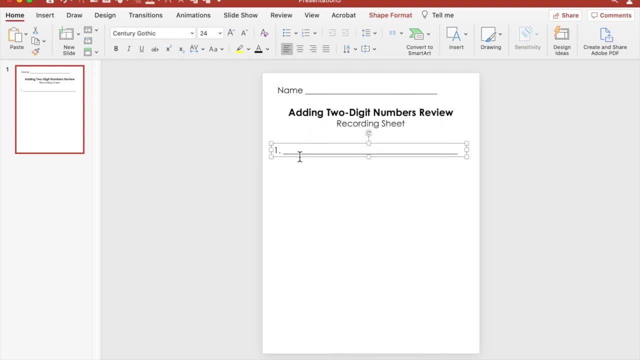 and then I'm going to duplicate it. Well, actually you can't duplicate it this way, But with your keyboard I'm going to press Command D, because I'm on a Mac, you're on a PC. just put Ctrl D And. 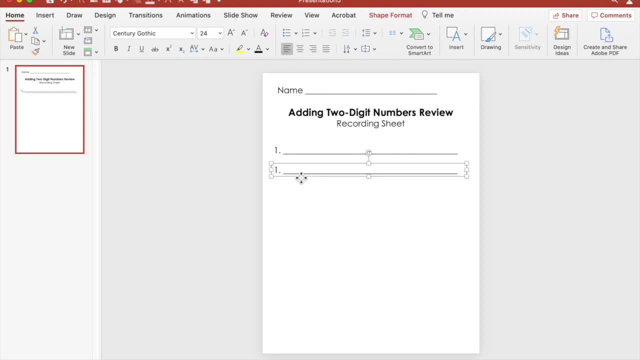 then I'm going to duplicate that and then place it under the first question in the amount of space that I want, And then I'm going to hit duplicate again, again, again, for as many questions that I want. So I think that looks good. 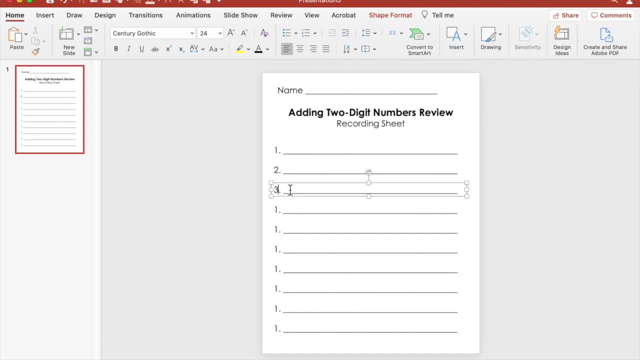 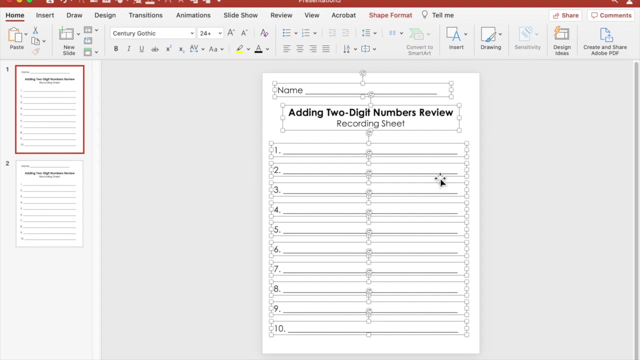 All I need to do is go in and change the numbers. That looks good. Let's bring this in a little bit. So there's our first recording sheet that we have. let's duplicate the page first so we can modify, and then I'm going to group by right after I. 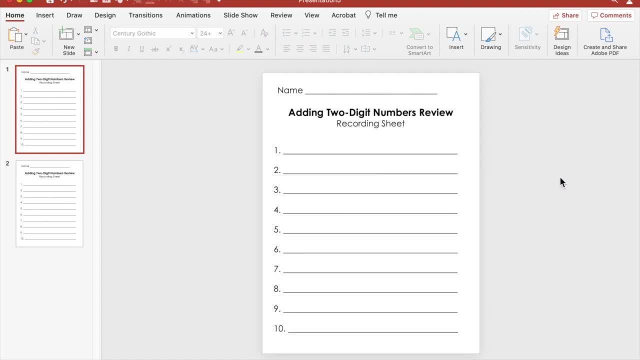 selected them all, right click, go to group and then group again, and then they're set together. So on this next one we're going to keep the same heading. But what if you wanted more questions but less of a line for their answer? 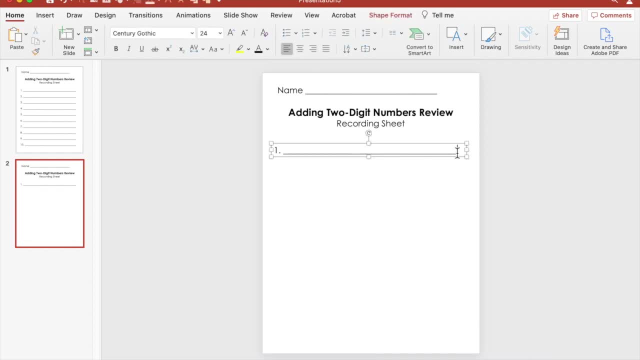 So I'm going to get rid of those and then adjust the line here. for the number one, that's a good amount of space. we're going to bring our text box in And then we're going to duplicate that text box And this time I'm going to put it here in the middle and then duplicate it again. it looks a. 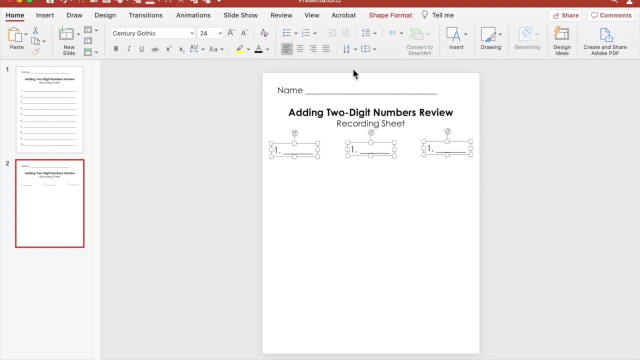 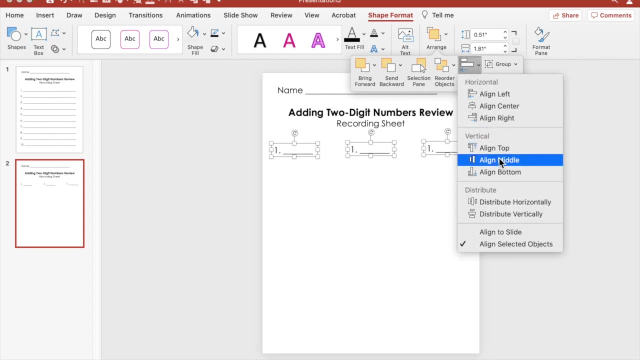 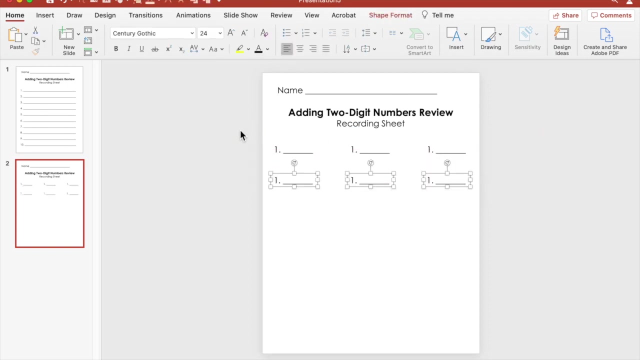 little higher So they're aligned. I'm going to select all three. go to shape format arrange. I'm a line, a line middle, so then I'm going to select them again and then duplicate, and then I can duplicate that row or I can take all of them and duplicate. 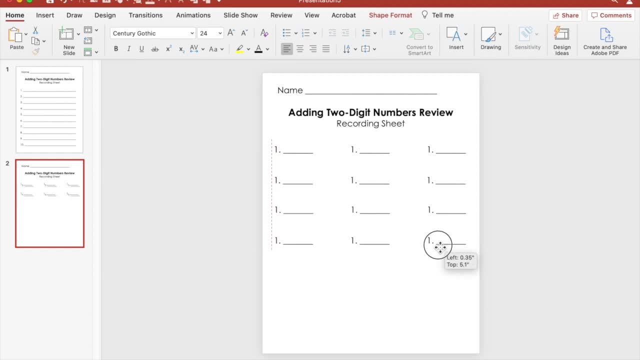 and then I'm going to duplicate one more time. I think I want more space between them all, so I'm going to go back to the first duplicate duplication. so I just undo. I hit undo many times to go back. so let's get rid of these and then select this and hit duplicate one more time. 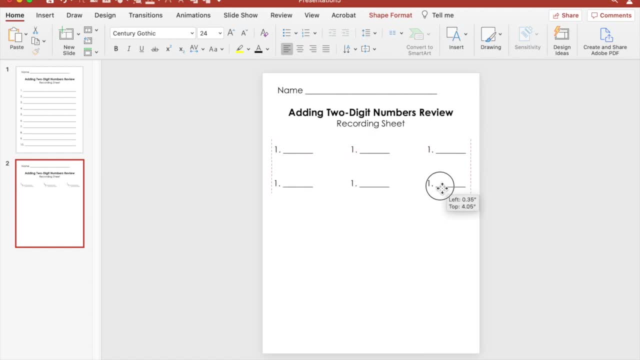 let's do there and then duplicate that set, and then duplicate that set, all right. so now we're just going to adjust our numbers, all right. so here's a tip. so once I got to the two digit numbers for problems, it made my text box overflow so that the line went down to the next space. so I want to extend the text box for each. 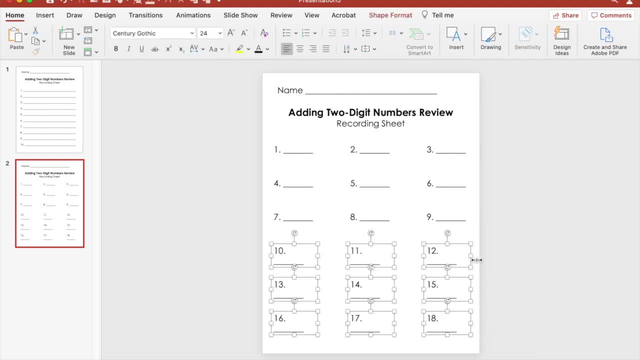 of these, so I can do them one at a time, or I can select them all and then just extend on one, and then it applies to all of the ones selected. so there you have, our second page recording sheet. so then let's do one more option. so I'm 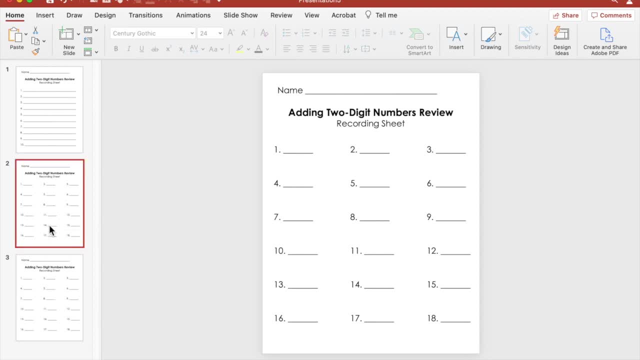 going to duplicate. I duplicated that page, so back here I'm going to highlight everything and then group them together because I'm done with this page. and then, on the last one let's get rid of, let's get rid of all of our text boxes. we're going to insert a shape and I want it to be a curved. 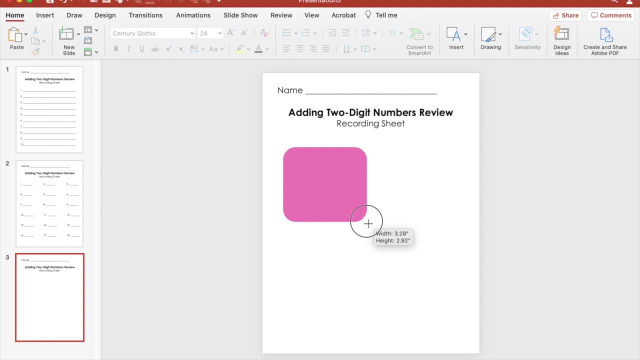 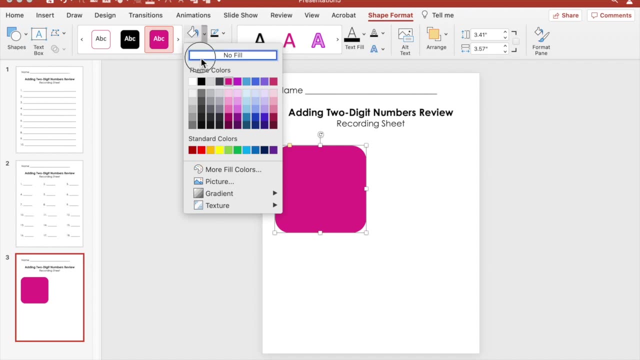 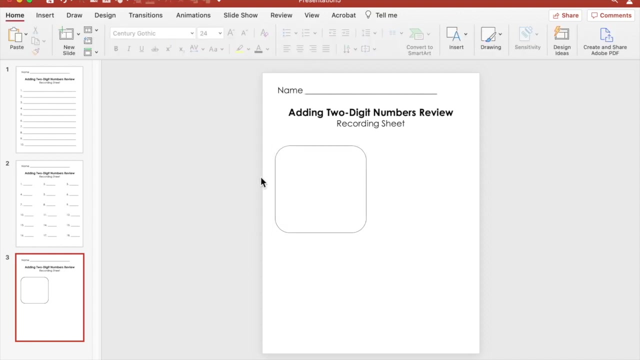 shape or a curved line. all right, so now I'm going to go up here to shape format and I'm going to put no fill, and then for the line, I want it to be black. you can make your line thicker than that if you like, and then I just 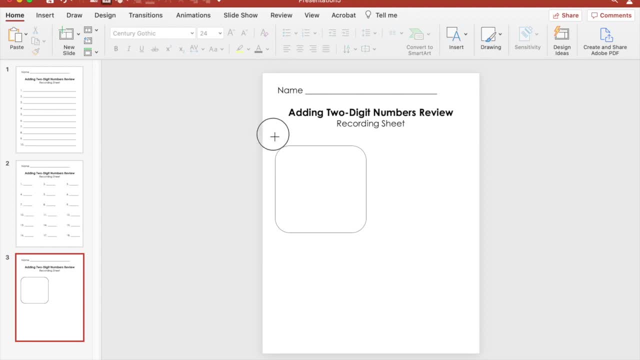 want to add in a text box for the number, and we're going to. you can leave the font, change the font, it's up to you now. put number one Center, bring it in, and then I'm going to actually put mine inside of the box for the square, or you can leave yours outside, whatever pleases your eye. so I'm 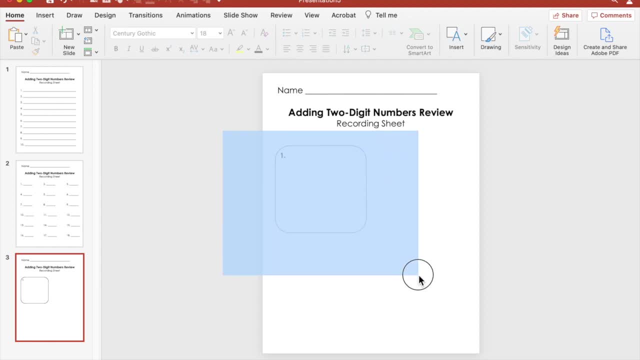 going to put mine in there and then I'm going to select both of them together and group, and then I'm going to duplicate it, bring it over and then change the number, and then I'm going to select both and then duplicate those and then bring it. 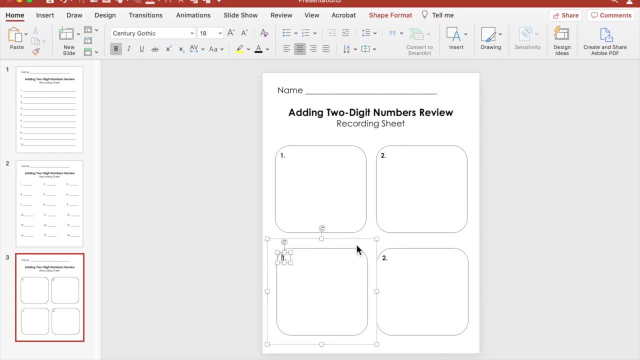 down and then just change my numbers. and there's our third example of a recording sheet. you can do a variety of things in a variety of ways with recording sheets, based on the needs of the task or activity you're having your students do. so the last thing we need to do is save our PowerPoint, and we're going to save. 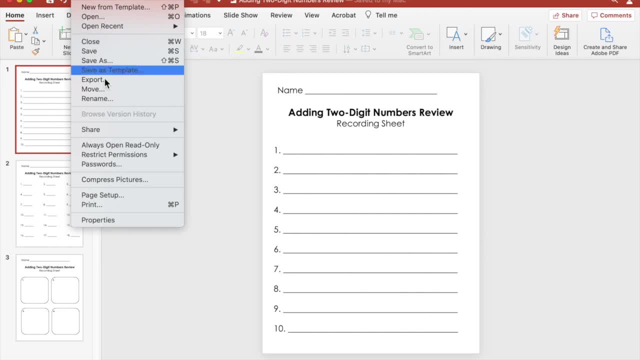 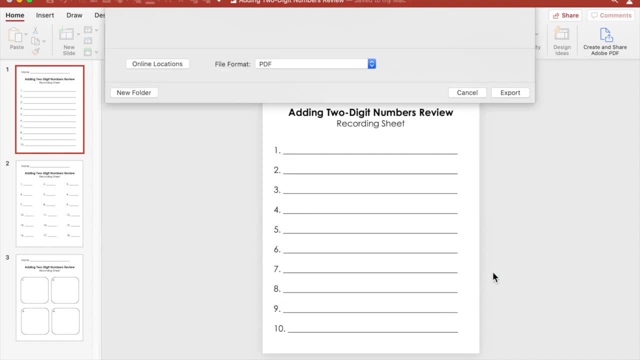 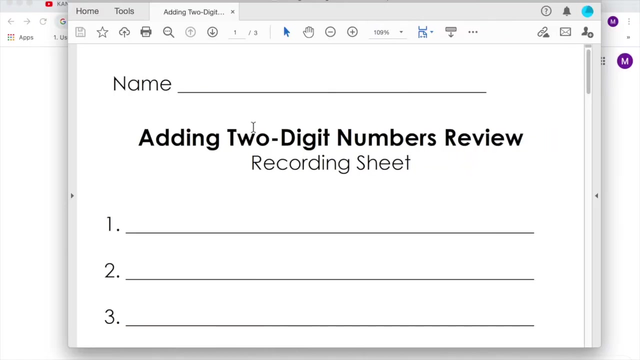 that. so then I'm going to go to file and export it as a PDF, remember? the title stays the same, it's just the PDF now and then export, export. I'm done exporting. I'm going to pull it up in my folder and look at it as a PDF. 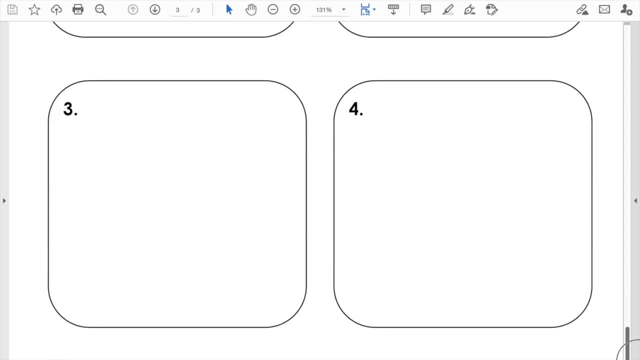 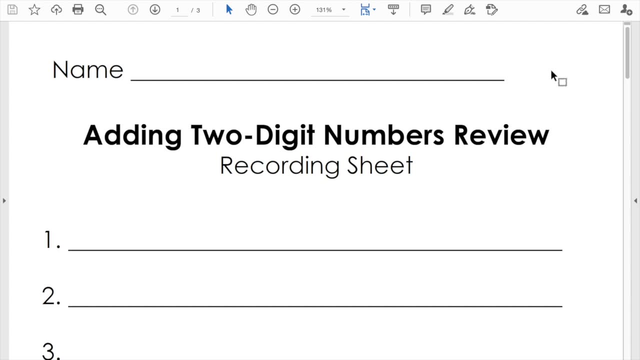 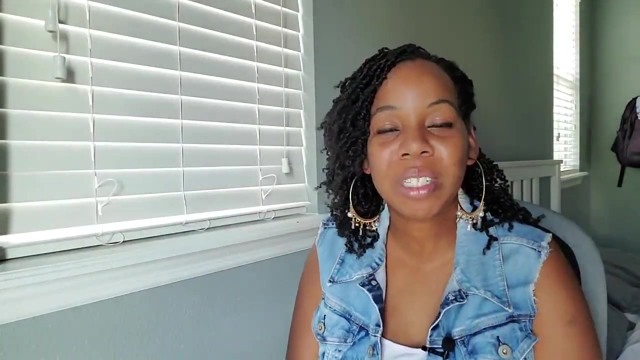 And then get ready to print it out for my students. I hope this tutorial helped you with learning how to create your very own recording sheets using PowerPoint. Okay, day nine is over. Now you know how to create recording sheets. You can add that to your math resource toolkit. And remember if you want to make your recording sheets digital. 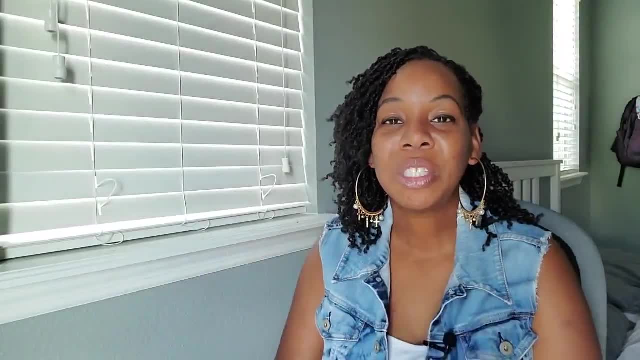 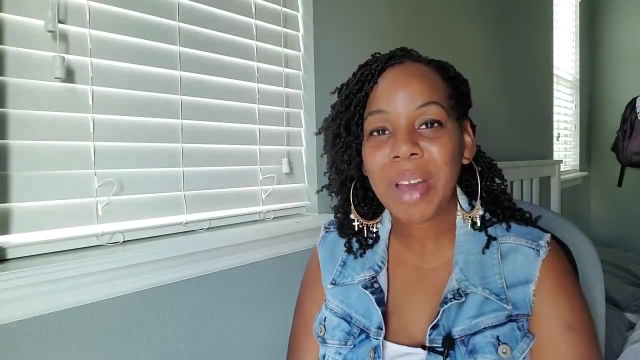 check out this video here on taking your PDFs from printable to digital in minutes. If you found this video helpful, please like it by hitting the thumbs up button, share it and subscribe to my channel, And if you want to be notified the next time a video is posted, please hit that notification.